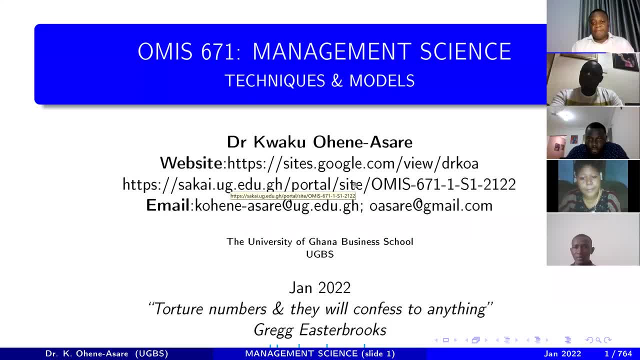 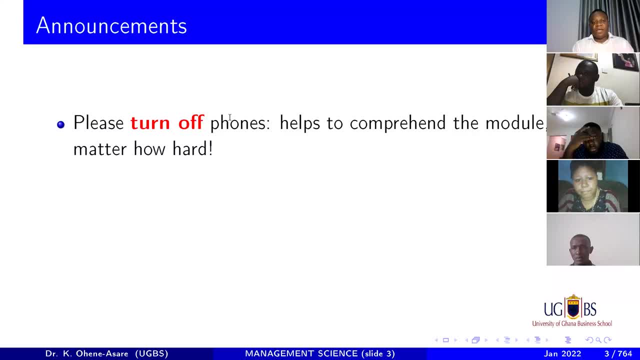 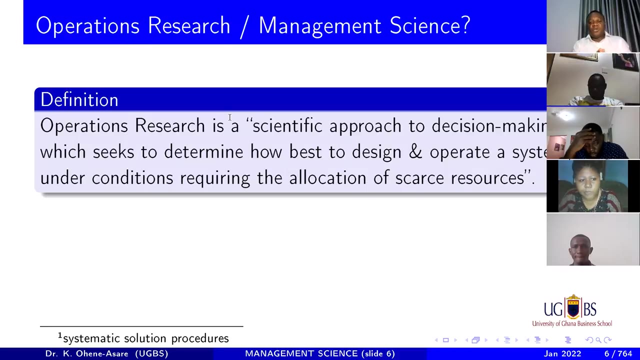 I'm going to quickly go through the housekeeping, because I've done this in another one. I welcome each one of you. Email me normally quickly. When things are not really doing good, quickly email me and then I can attend to you. I want to start by telling you a little bit. 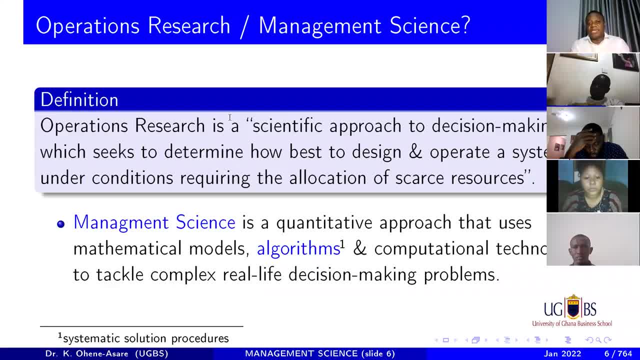 about management science. Management science is also known as operations research. It's a scientific approach to decision making. It's a quantitative approach that uses procedural analysis, algorithms, mathematical models, computational techniques to tackle complex real-life situations. If the situations are not complex, you see that if situations are, 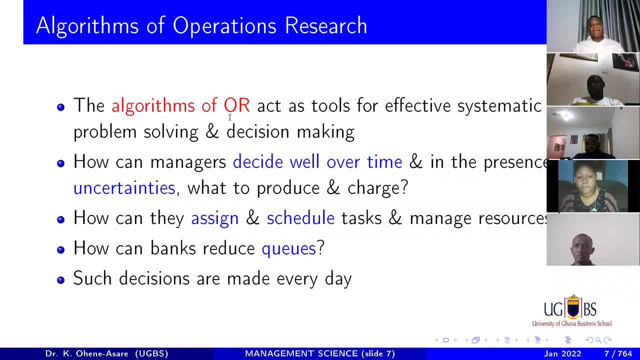 complex people are not able to handle it well. Management science can act as tools for effective dealing with systematic problem solving and decision making analysis. For example, how do you decide ahead of time, in the presence of uncertainties, what to produce, how much to charge, how much profit to generate, How? 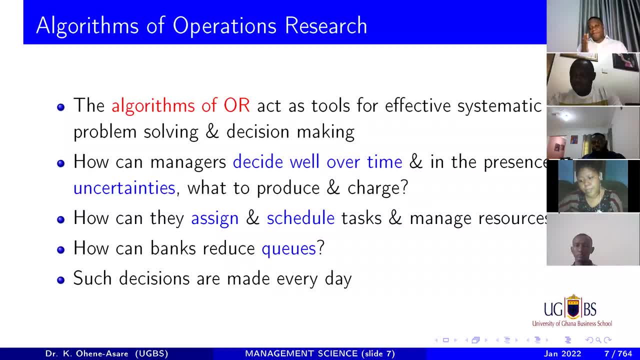 do you assign workers, schedule a task for them so that you'll be able to now do scheduling? Okay, How can you reduce queues in bands when students are registering in voting time? How do you reduce the queues? There's something known as a queued model. You shall look at that. 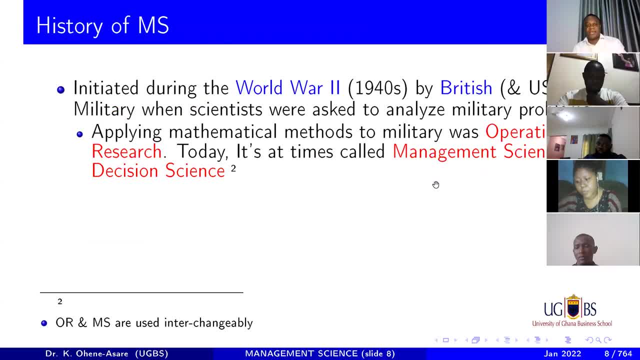 So these are things that happen in real-life businesses. And the last time we indicated that management science was born out of operational research or operations research, It was born out of operational research and research. It was started in the Second World War, where the British 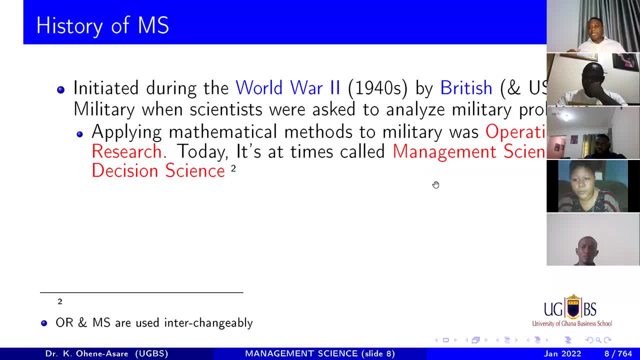 and American military devised strategic means to win the war. They set up strategic moves, strategic models to win the war And those methods, those strategies, after the war became much more applied in engineering, manufacturing, health, business, telecom And today. 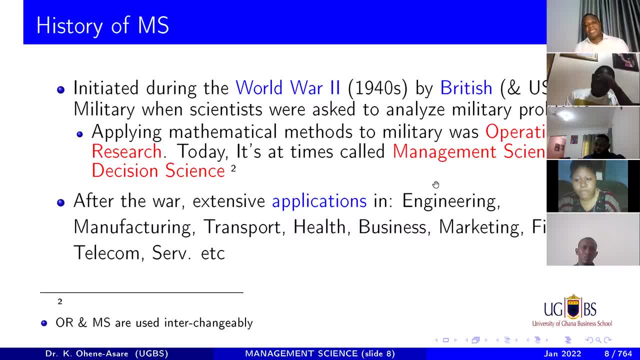 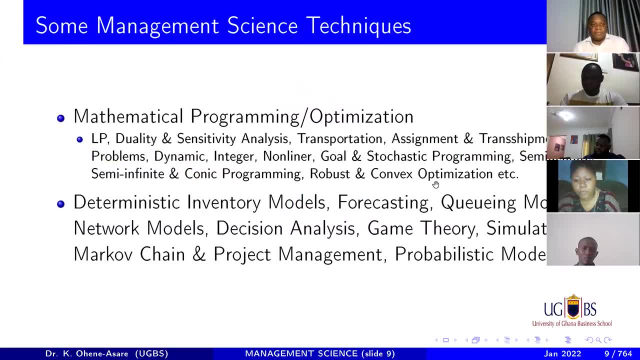 we study these things in management schools And it is collated to be known as management science or decision science, as we know today. So management science uses techniques, methodologies, to be able to simplify complex things so that man can handle them. Some of the models are the techniques that management science deals. 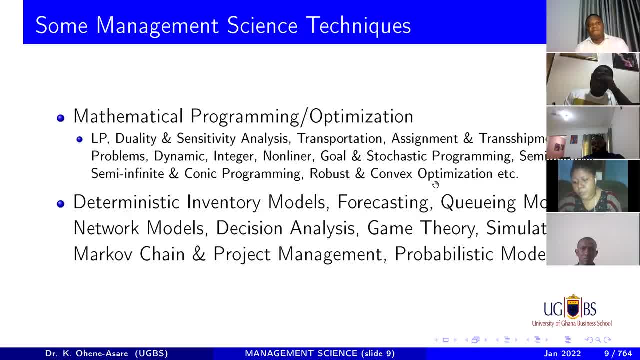 with are different aspects of mathematical programming. So we shall do a lot of this. We shall do linear programming: duality, sensitivity analysis, transportation, assignment, transectment models. Next semester you'll be dealing with dynamic integer linear programming, goal programming, stochastic programming. 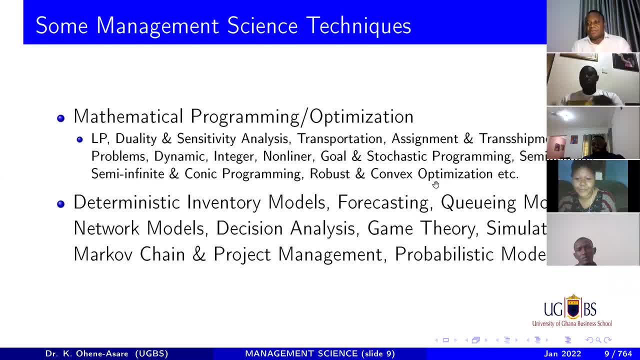 some infinite conic programming, robust optimization, Welcome, Welcome. If you were telling your family members, you are about to study operations. now is the time to prove yourself that you are about to study that. We shall look at deterministic models. We shall look at forecasting in this world, human models. 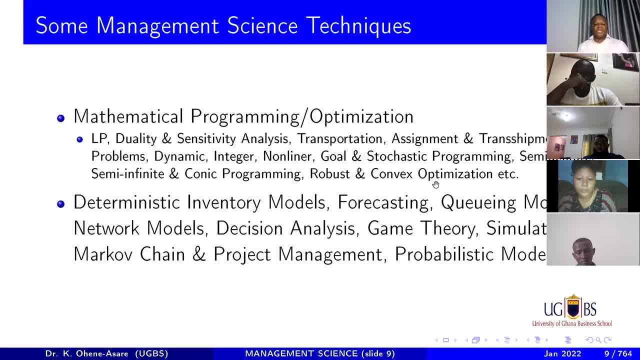 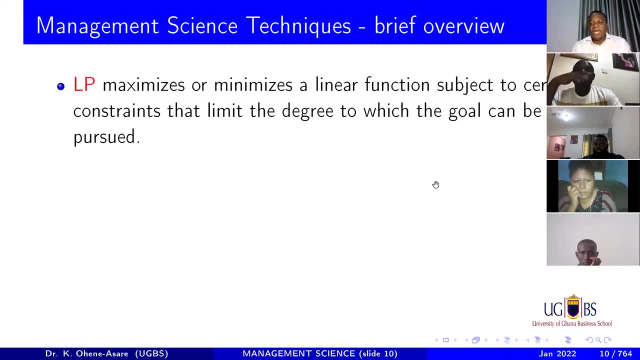 network models, decision analysis, game theory: I'll teach you game theory. I will not be able to teach you simulation. Markov chain probability: I will not be able to teach you probabilistic models- Some of them. you study them next semester. 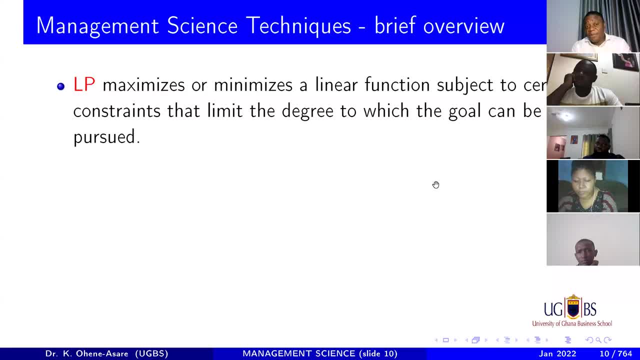 So let's take a brief overview of some of these. The linear programming we are going to do today, so I will not dig deeper into that. Queuing models: they help managers understand the best way to reduce queues. So what it means is that by the time you finish this course, 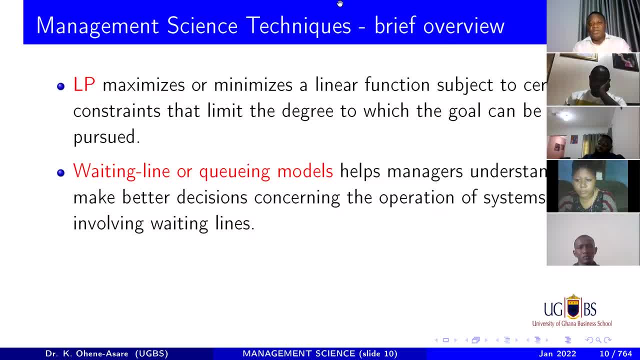 you can be able to reduce, develop a model that is more efficient. So let's take a brief overview of some of these things. The linear programming is a model to reduce the queues That build up in your company or in any particular company. 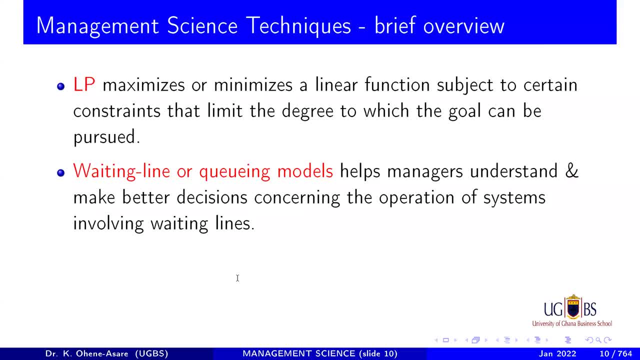 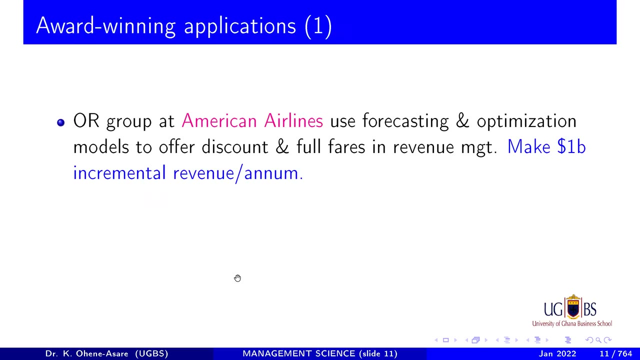 DEA is a data envelope analysis is a linear programming frontier methodology for assessing the relative efficiency and productivity change All firms that are similar in producing output using some. We shall study this fully. second semester. Sometimes people wonder whether management science, decision science or personal research. 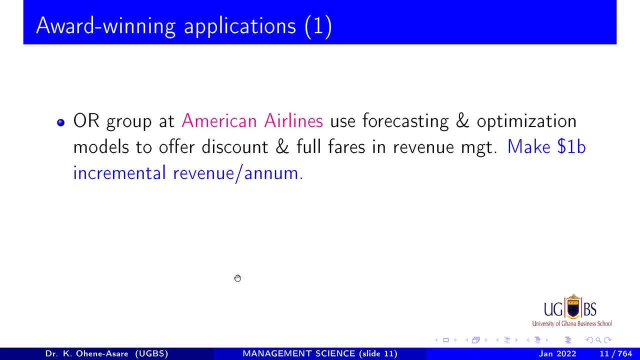 whether it is real, whether it can be applied in real market systems, and I guarantee you it can, It can, You can apply this thing in real life situations and I'll be asking you some of this when I'm done. For example, the American airline as we know them today. some years back they were able. 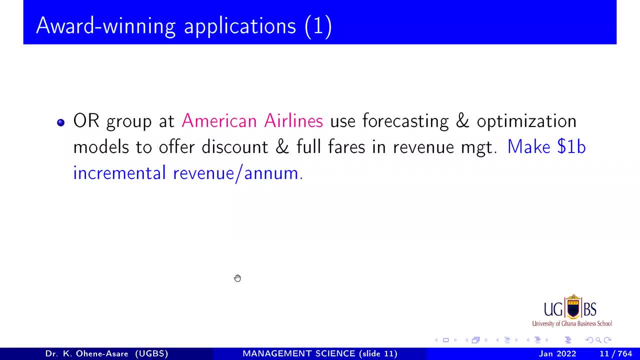 to use forecasting and optimization, both of which we are going to study. They developed these models and used them to offer discounts and full face in revenue management. In the process of doing that, by one year they made a billion dollars in incremental revenue. 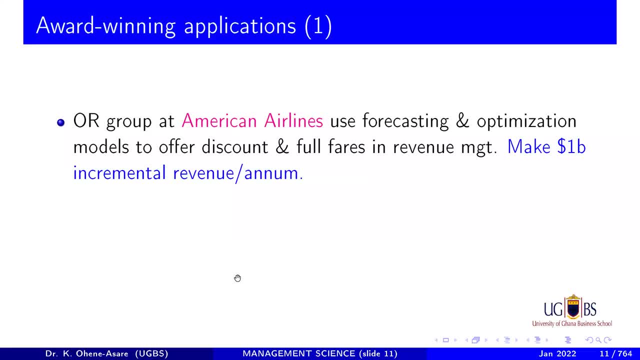 One billion dollars Just by adopting the method you are about to learn in this course. So who says it's not applied And who says it is not, you know, useful? There's a lot of money in there. China: they are well known when it comes to projects. 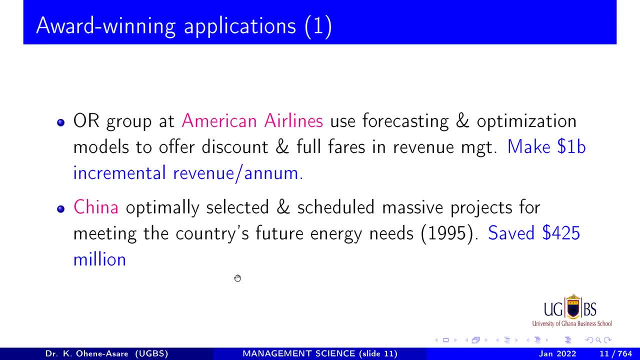 They build a lot of big, big time projects. Now they wanted to handle their energy need because China is a very big country, over a billion people, And energy has been a concern. In 1995, they used optimization scheduling and they were able to use that in their energy. 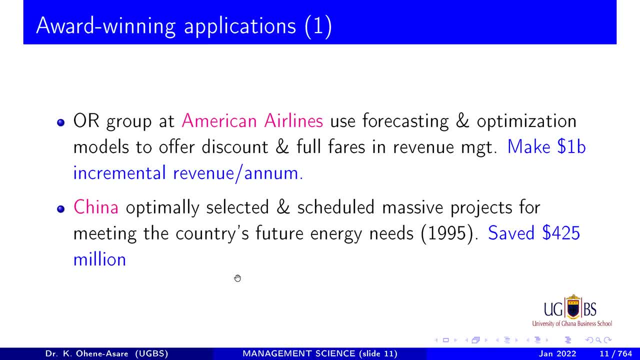 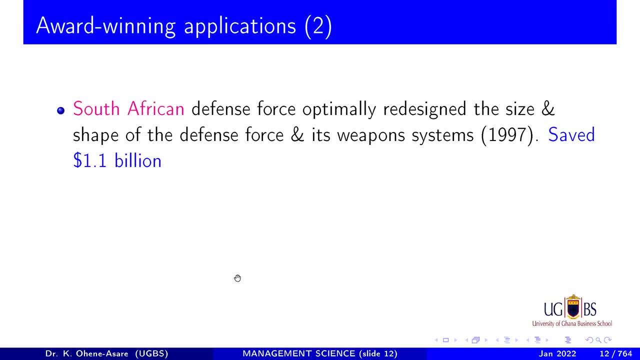 needs and they saved $425 million. The cost, the methodology that they used is what you are about to learn in this course. South Africa in 1997, just some few years after the apartheid regime. They had a demand. They had a demand. 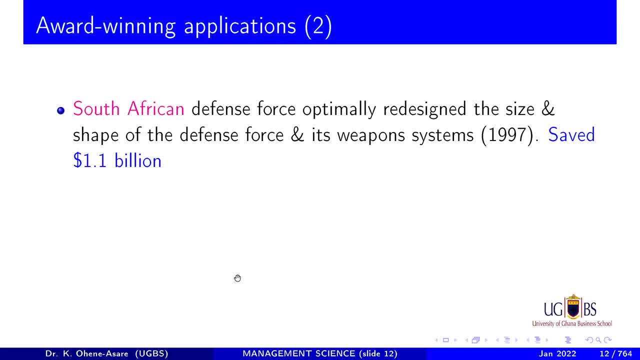 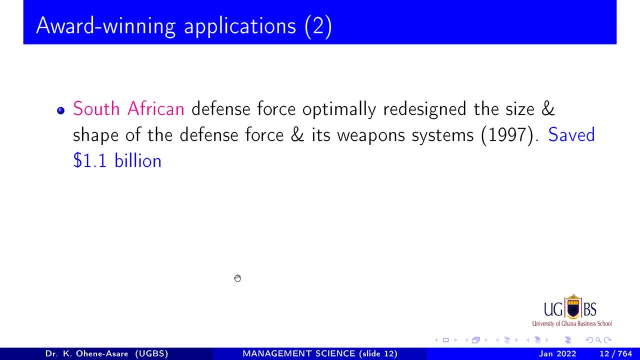 they sometime tools. the Z Explain the price. They solve the deficit growth. Tuesday earlier, Pristons and Alkaroo smile Best use form of energy switching. They are the defense force And they optimizing, redesign the. a Vaigna or the ship of the defense, worried. 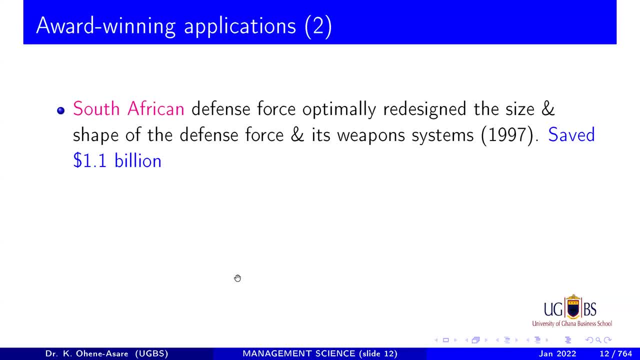 And the entire. what proteins Systems, They're redesigned And the use optimization. They said $1.. say $1.. picture with: I think I'll go again 1. Billion dollars, Just using the technique you are about to study. 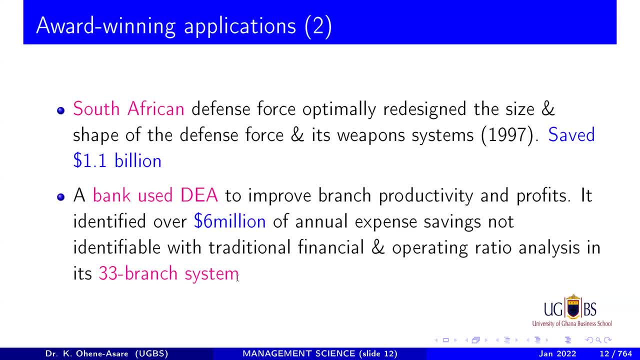 If you agree with what you say. we argue that they have first hand and the semester. I know a particular bank myself in California. the bank had 33 branches and they used data envelopment analysis, which is one of the techniques you'll be learning next semester. 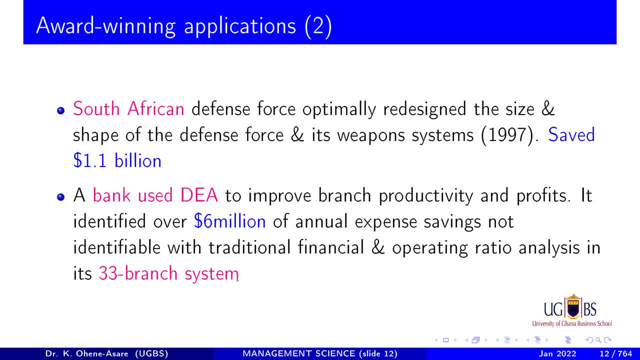 They used DEA to evaluate the relative efficiency and productivity of the branches of the bank, and in one year they were able to save $6 million That were not identified using traditional financial and accounting ratios, and so it goes to show that, beyond accounting ratios, something else can bring about, you know. 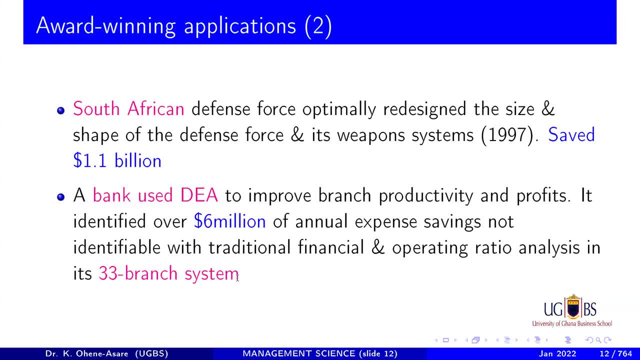 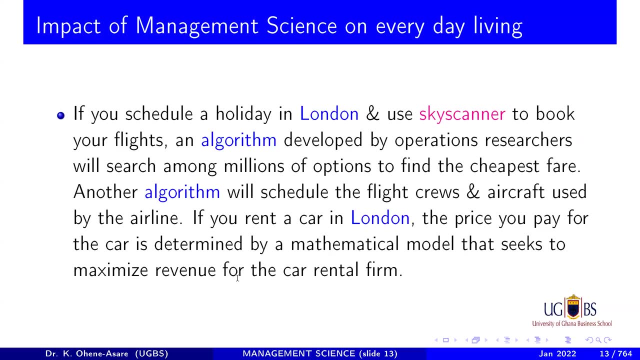 efficiency. Are these not telling information that shows that management science, operational research, is very, very important to businesses, society and individuals? But let's get even funny and look at a practical demonstration of management science in your everyday living. in your everyday living. 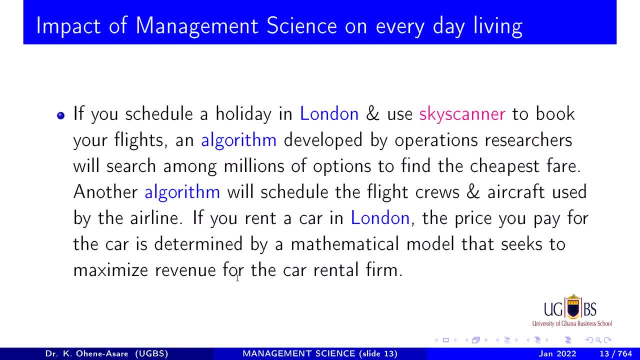 Let's assume that you want to go on a holiday in London, and normally you will go and search for the cheapest flight, and so you use a sky scanner. Those of you traveling you know it: You use a sky scanner, and the sky scanner has several algorithms. 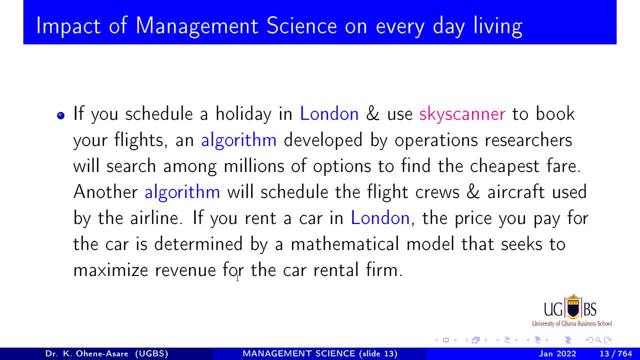 It's just like Google. okay, Larry Page and his colleagues. they developed several algorithms in which, if you are able to say what is phantasmagoria straight away, Google has an algorithm that will immediately search the entire world wide web and will fish out that. 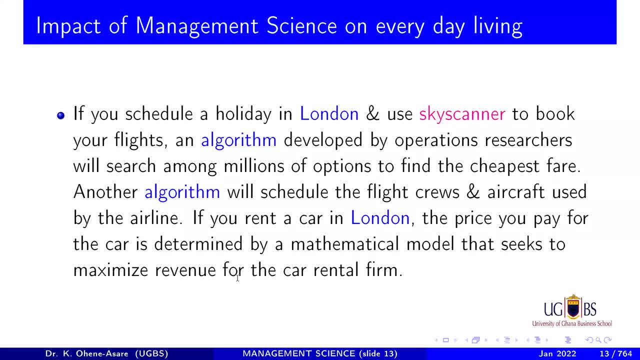 Okay, It will give you multiples of areas where you can find the meaning of phantasmagoria. So the algorithms that have been set up in sky scanner will find the cheapest flight for you, okay, the cheapest fare for you, and then you'll be able to now get it. 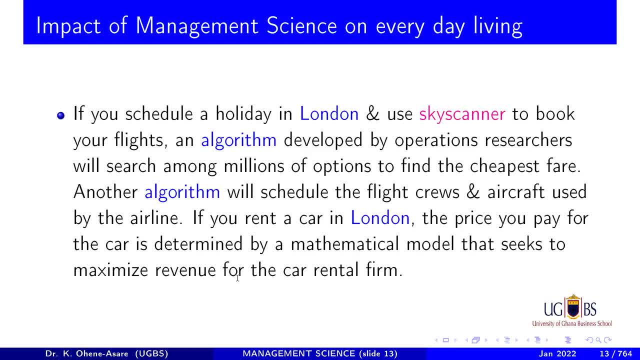 But then you can also use another algorithm that will also schedule the flight crews and the aircraft that are used by the airline. You can see that, If I can use it, the algorithm even helps you to be able to know which seats you want to sit on and whether that seat is occupied or is not occupied. 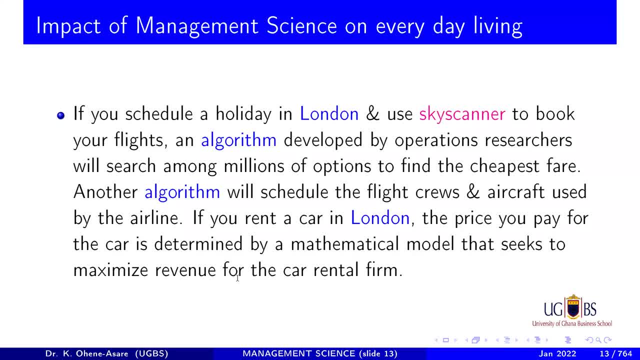 All of this. you don't see it all, but behind the scenes things are happening, Procedural analysis are happening, And if you were to go to London- and probably you need to rent a London cab- that will take you to your final destination. 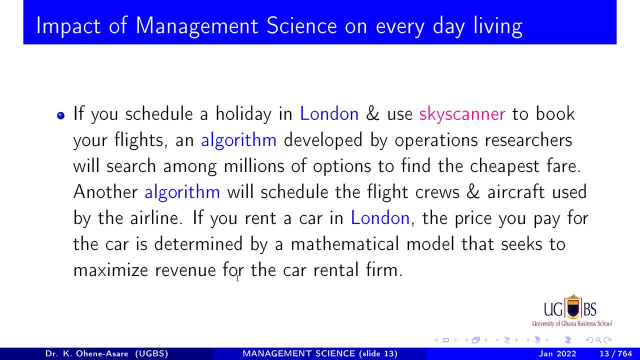 The price that you pay to the cab company, that black cab company, that price you pay is determined by a mathematical model And that model is designed to maximize the profits or the revenue for the car rental company. Management science is at play. Management science is happening. 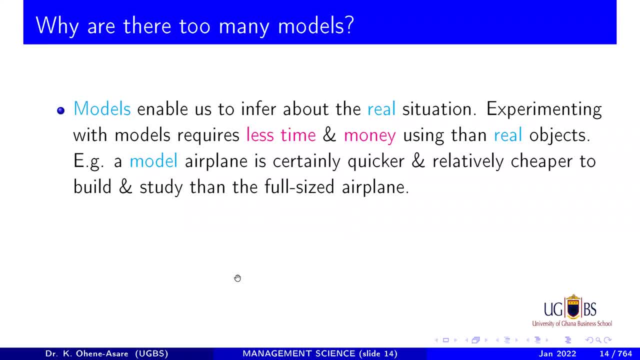 And so who says that is not practical? But if you want to go ahead and do it, you can do it. But if you want to go ahead and do it, you can do it. And so who says that is not practical? But if you want to go ahead and do it, you can do it. 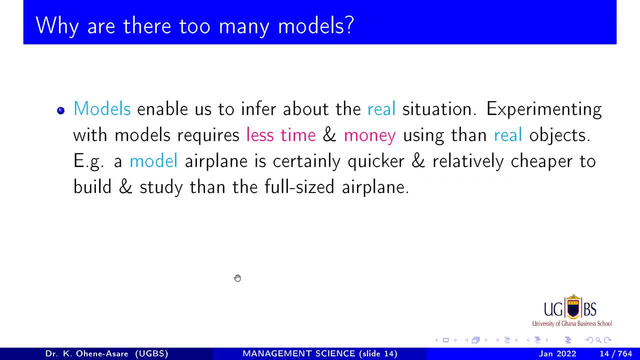 And so who says that is not practical? Because you may run into the real life like this. It's not going to be easy because the real life things are complex. So we use models in management science. So in management science you will be experimenting with models. 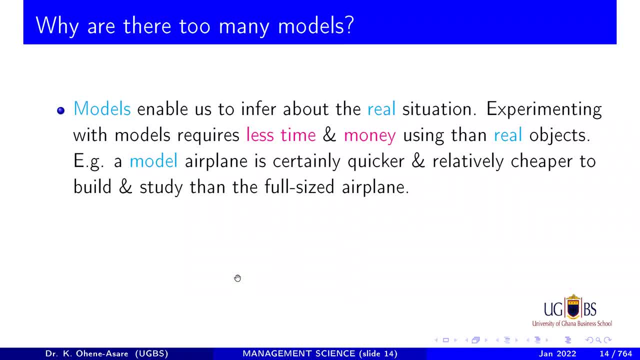 But models will save time because you are not dealing with a real artifact. The models will also help you to be able to cut down costs And you will save a lot of money. For example, if you have a model of an airplane, You can manipulate the model of the aeroplane to know whether to have an accident, simulate it, bootstrap it before you can deal with a real full-sized aeroplane. 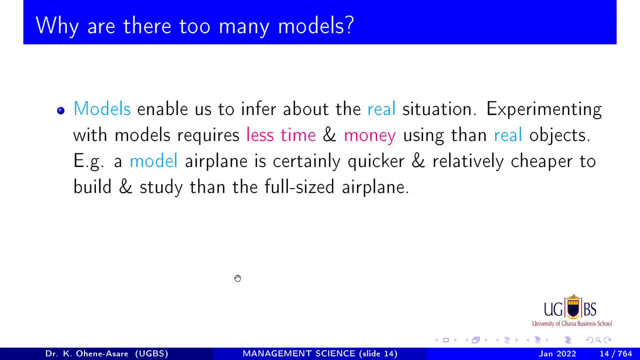 But if you want to deal with a real full-sized aeroplane straight away, it's not going to help. So in management science, we use models or develop models or enhance models. Ladies and gentlemen, you'll be building models. For the first time in your life, you'll be dealing building models. 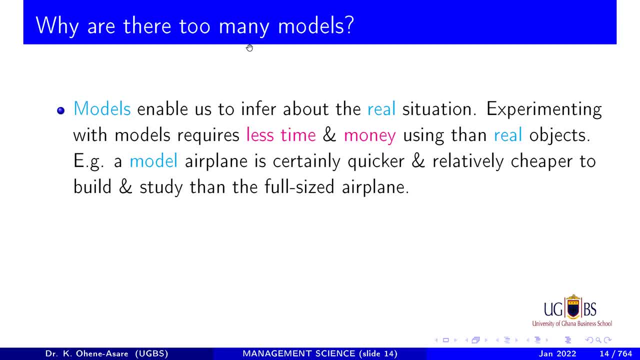 Let me ask you whether you remember these things in your secondary schools, or A-levels, O-levels. Do you remember the days when you used to do simultaneous equation? word problem: If you remember, just type yes for me. If you don't remember, just type no. 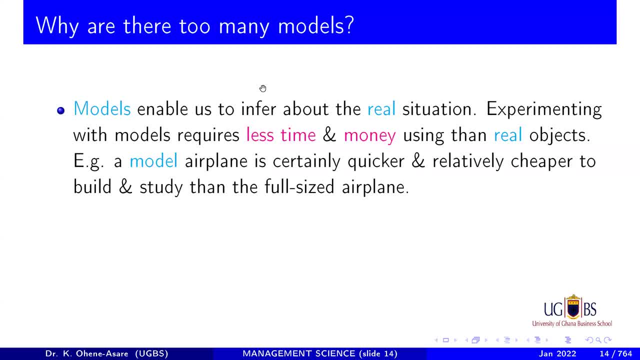 Do you remember the days when you used to do simultaneous equation word problem? Do you remember the days when you used to do simultaneous equation word problem? Coffee is two years, five years ago, older than his father, Younger than his father. His father at the time was 60 years. 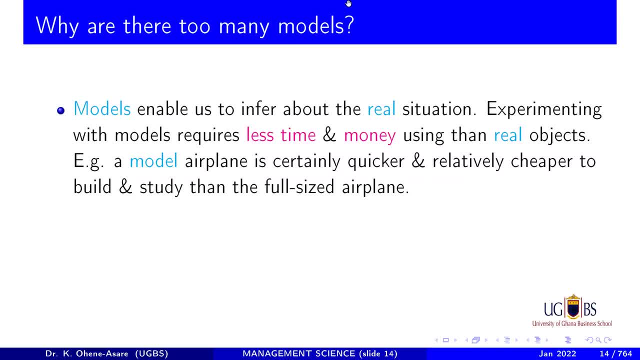 But his father was seven years older. You know those kind of things. That's it. That's it, That word problem. when you have that word problem, you have to convert it into a simple word model. Okay, a simple model. and that model can now be manipulated to find the answers to that. 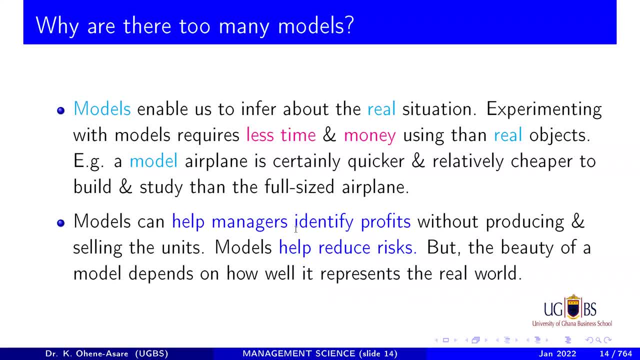 order. so models are very good. they help the managers identify profit and revenues and reduce the risks. you know, but if you give a wrong modeler, you're going to get a wrong solution, so your model has to be correct. if the model is wrong, the solution will be wrong, so we'll 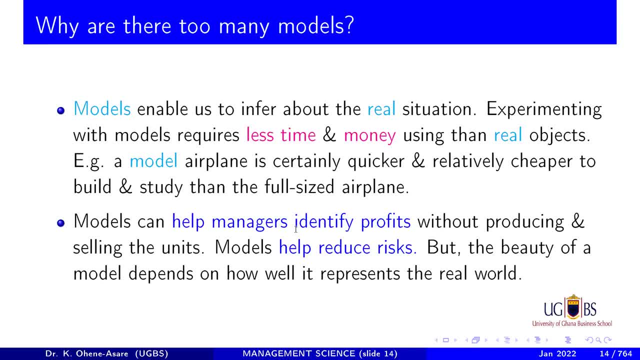 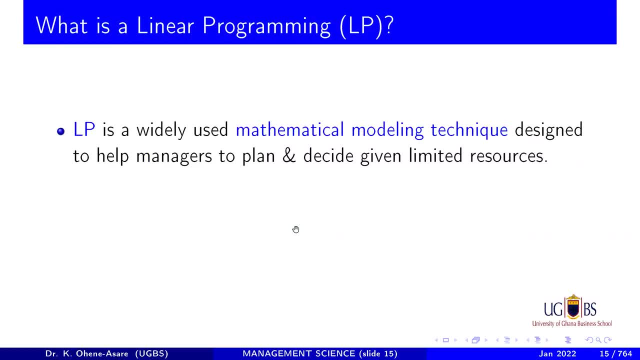 be dealing with models that are sensible models, so that it can represent or mimic the real world. so we're going to look at one of the first techniques, and this technique is going to take us about three weeks to one month to complete it, because it's detail is probably the most. 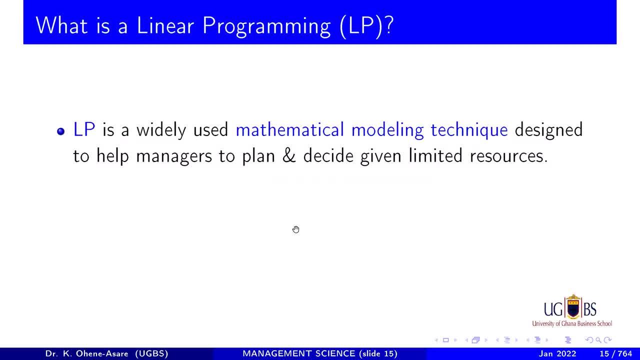 important technique in management, science, operations, research, and that is linear programming model. linear program, or lp, is commonly used mathematical model designed to help managers decide ahead of time how to maximize their profits given the limited resources at hand. based on the linear program, you can develop scheduling, you can develop management. you know efficiency situation. 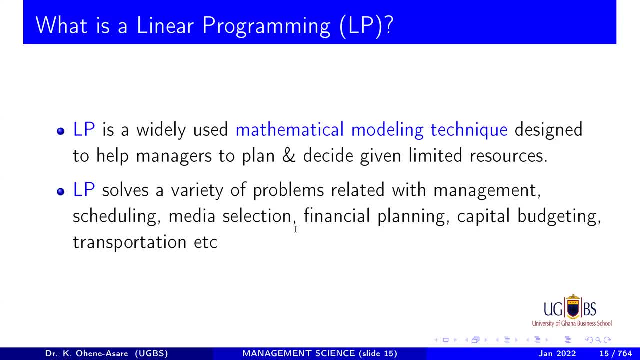 medium selection situation. in fact, you can handle financial planning, capital budgeting, which instrument of finance to invest in. you can handle how to shorten your distances. you have to travel to carry things from one place to another, transportation. linear programming can help be applied in all of these areas and, and that is what we are going to be looking at- where did it? 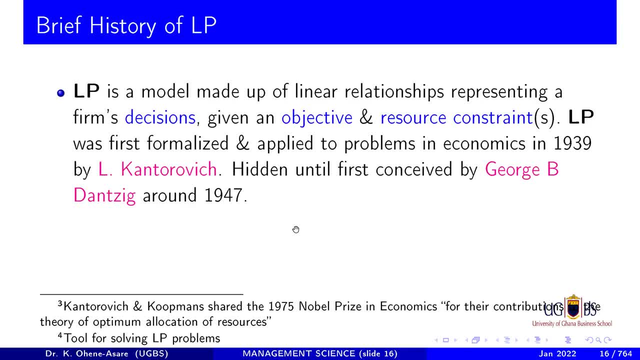 begin from it start started as a model. I'll look at the details, the components later, but it was first formalized and applied to in economics by a man known as Kantorovich. This was in 1939, but it was. 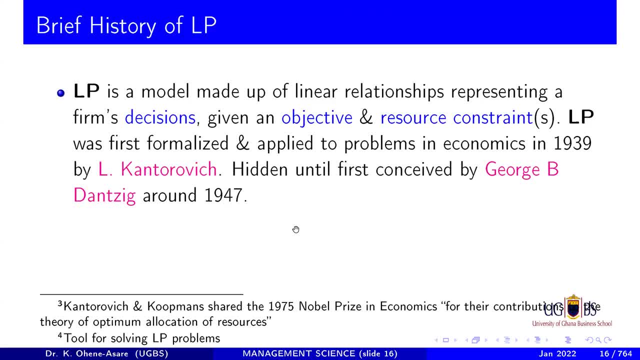 not popular until George Ganszik in 1947, during the war, Of course. right after the war, during the war, that was when George Ganszik developed the simplex method. That was the name of it. The simplex method was designed to be used as a way to deal with a linear programming. 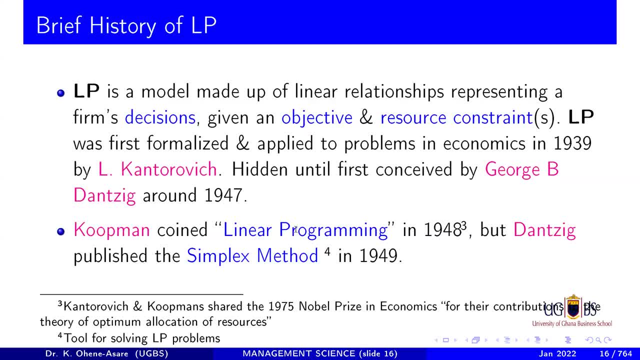 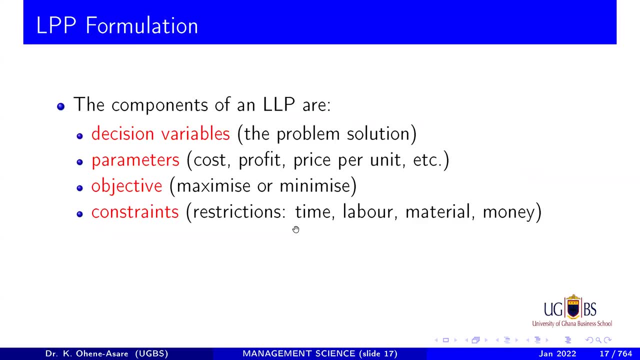 problem. These people have been well known to be great people in terms of Nobel Prize. That is how it began linear programming. It is attributable to George Ganszik. What are the components of linear programming problem? Well, the components are here. First, 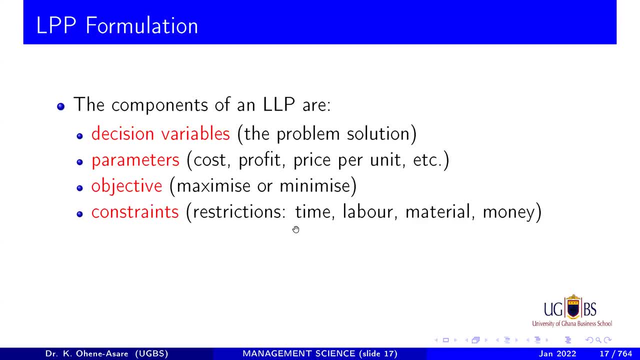 you need to know a decision variable, A decision variable. listen carefully, because this is critical. this is important. this is where you need to get into one. If you are going to go into any business, You've got to make a decision. 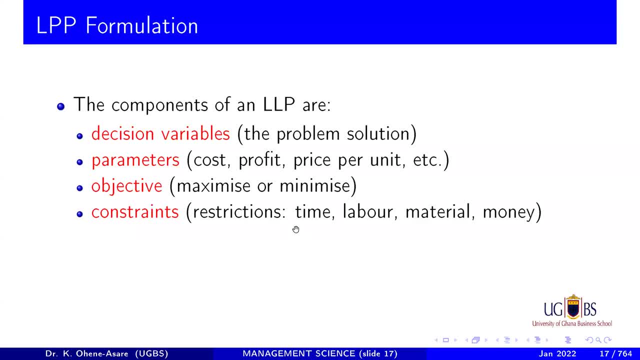 Decision on what you are going to produce or sell, or bring out or showcase All the services you want to produce. you want to be able to make that clear. You got to even decide the quantity of each one of those things you got to produce. you got to 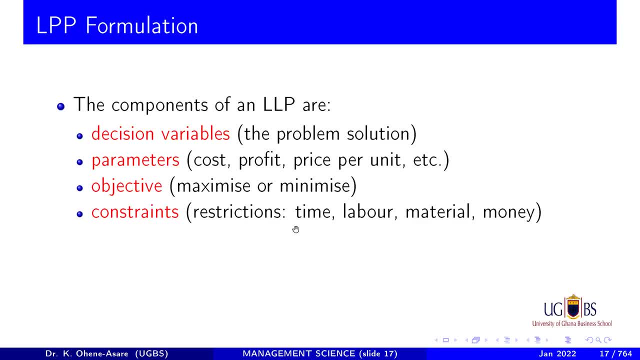 service got to give to people and That is your main problem. That is it. So when that is your problem, that is the linear for the programming problem, You're able to solve that problem in order to bring a solution to the problem. That solution to the problem is your decision where. 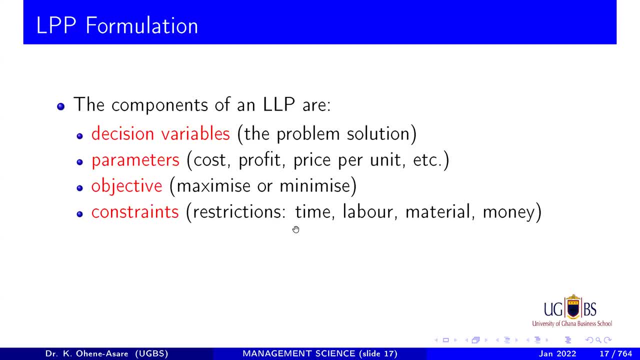 That's your decision variable. let's say, for example, you want to be able to go into the production of sheds, shots, pants. That's why you want to go into the production of. You got to know there, of course there's going to be some materials. 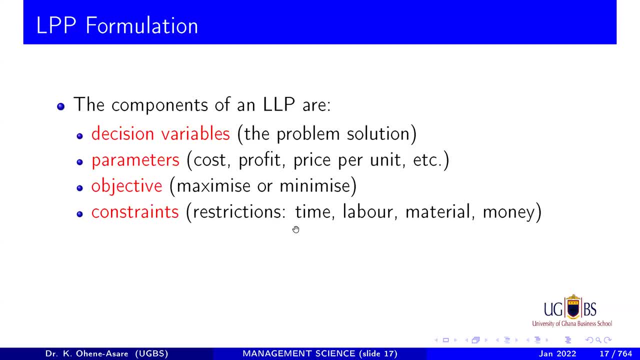 There are some materials you are going to use to do this production, But at the end of the day you've got to make a decision on How many of the shots, pants and then Sheds that you have to produce. So the decision variable Has to do with the item that is coming out. 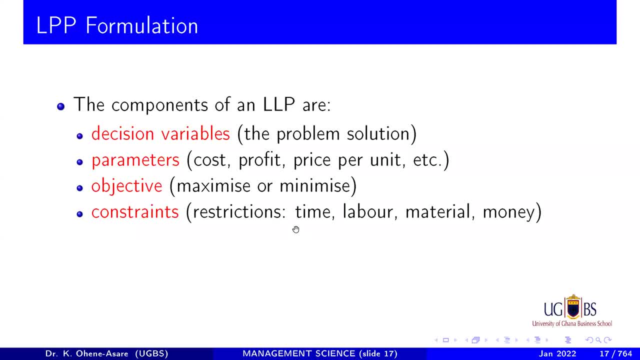 The quantity of those items That is coming up. I'll combine the parameter and objectives together and you will always have an objective, objective reader to maximize or minimize The overall, you know- output. now the overall comes from the decision variable multiplied by Its price, its coefficient. 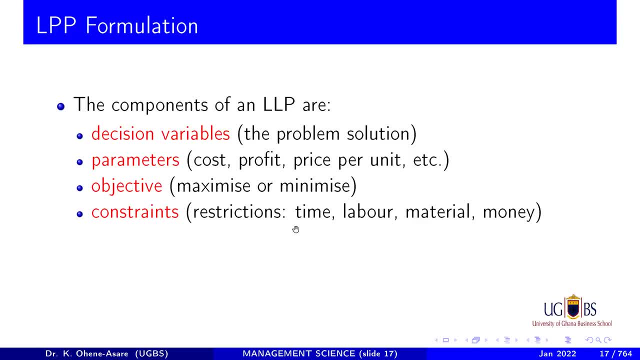 Or that item you're producing is per unit price. Your goal is to maximize That's, whatever outcome. so if it is sheds, shots, pants, and You represent each one by X, 1, X, 2, X, 3, Those are the items. but each item will cost something. So when you multiply the costs, 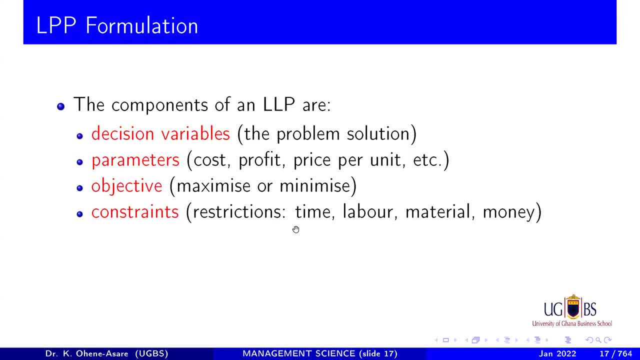 By the item you are able to get a revenue And, of course, if you have other things to deal with, you're able to Do some analysis and get profit out of it. That profit is the objective and your goal of that is to maximize that parameter profit. 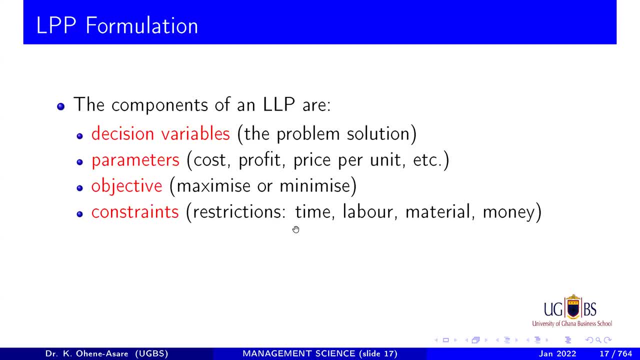 But of course it's not every time profit is Maximized. What do you think we have to do to revenue? Type it there for me. You don't maximize, We maximize profits. What about revenue? Do we maximize, Max or minimize many? 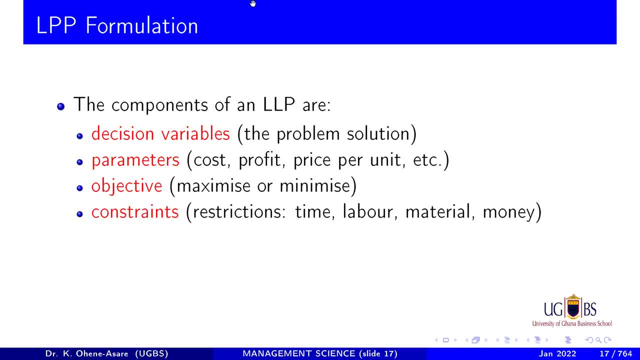 Revenue. Do we maximize it or minimize it? I'm checking those who are commenting with me a lot. Okay, Where could Richmond vendor? So you maximize that, you maximize Revenue. What about cost? What do you do with cost? Cost, Cost, Cost, Cost. 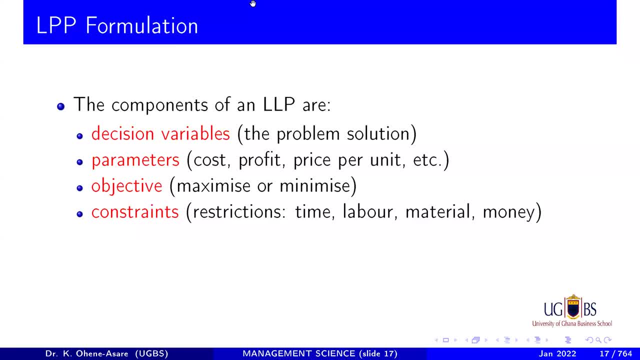 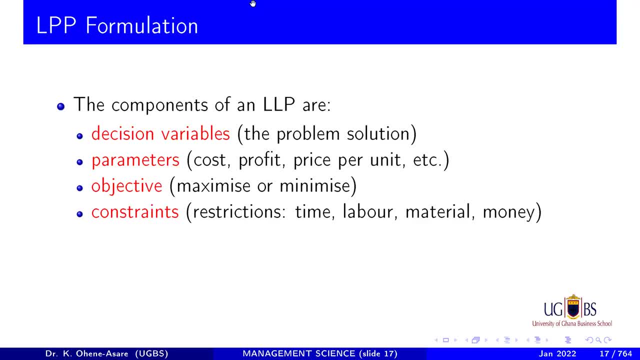 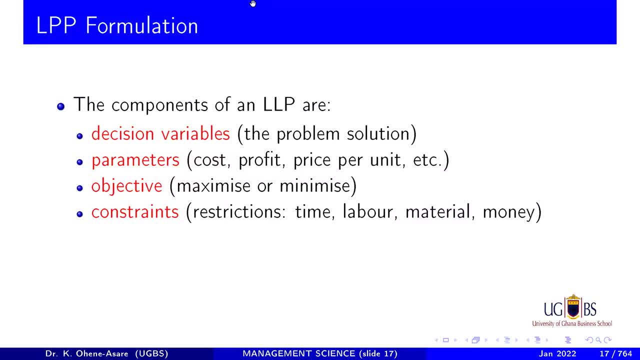 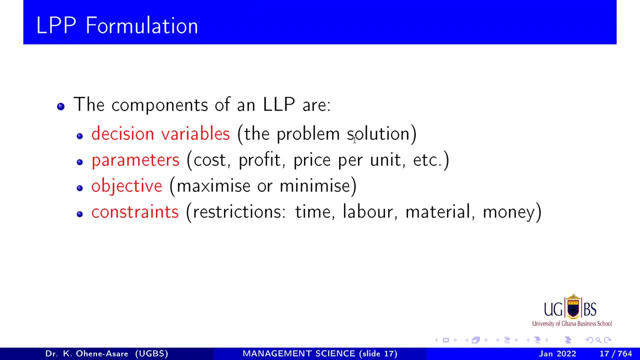 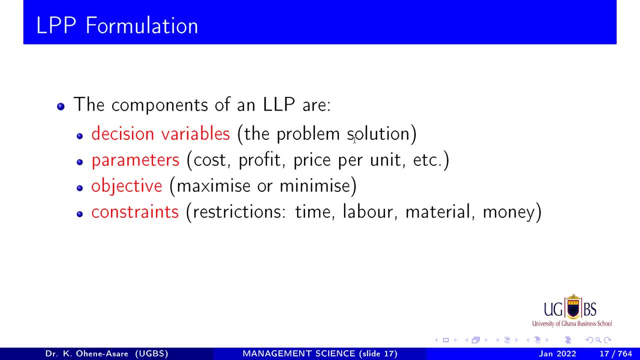 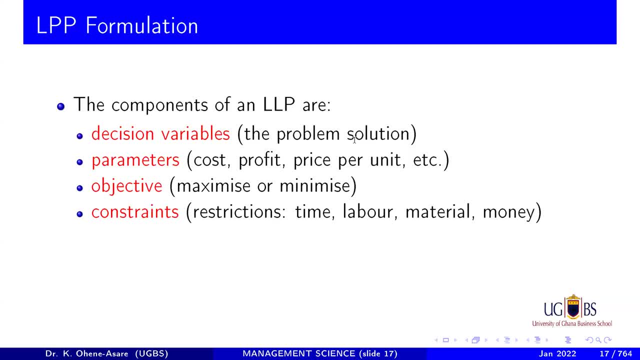 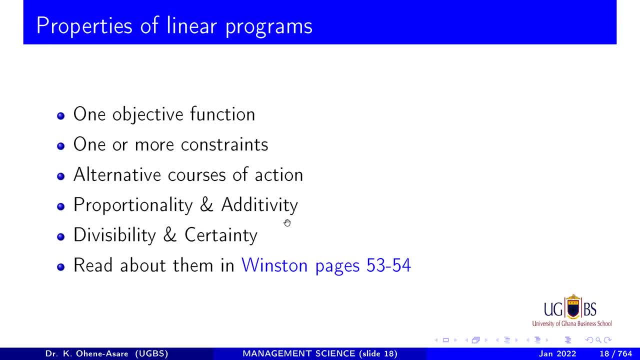 What do I mean by the properties? The properties are certain things that have to be there more or less for certain things to work, So they have to be there. They are one of the characteristics or features whenever you're undertaking a linear programming. 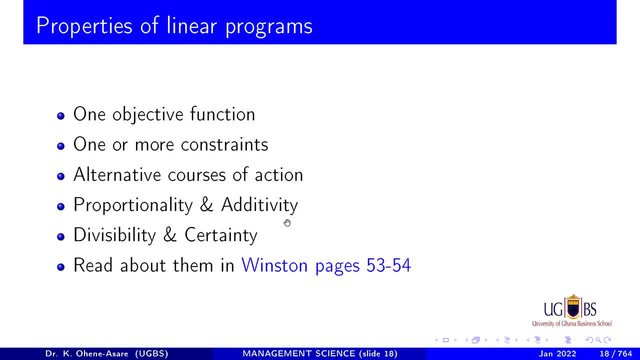 problem And one of the first properties to recognize that there is one objective function. It is not multiple objectives, It's one objective. In next semester you'll be dealing with multiple criteria, decision making, which is known as goal programming. That one: there are multiple objectives. 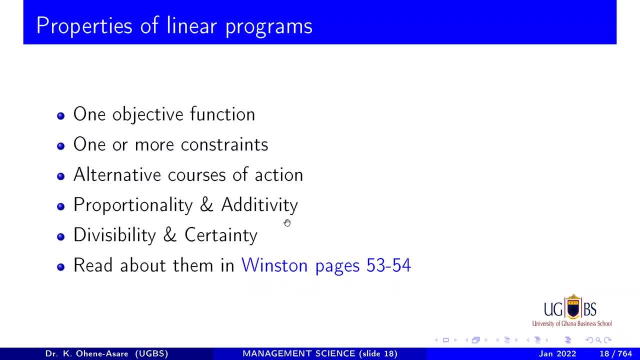 The second thing about a property. one of the features you note about this linear program is that you can have more constraints or one constraint. So the one of the constraints can be labor, capital, time and all of that. There are also alternative causes of action. 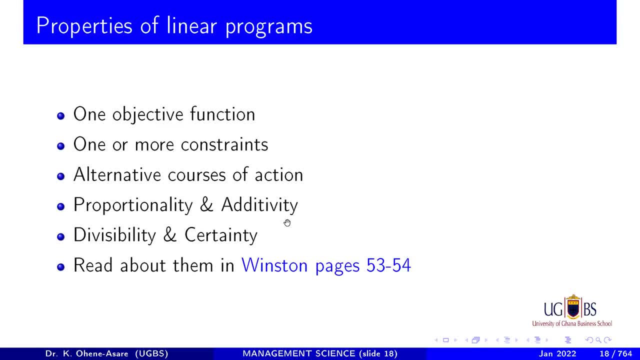 So it's not one cause of action you've got to deal with. There are several options, alternative causes of action. You will deal with proportionality. So proportionality means a percentage of this will lead to another percentage of that. So if you had to increase the labor by 20%, you expect a percentage of that 20% to reflect.